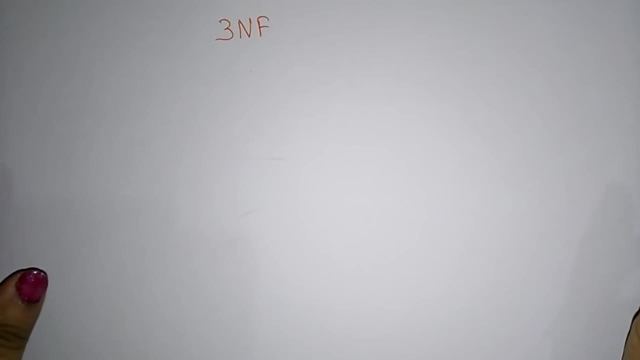 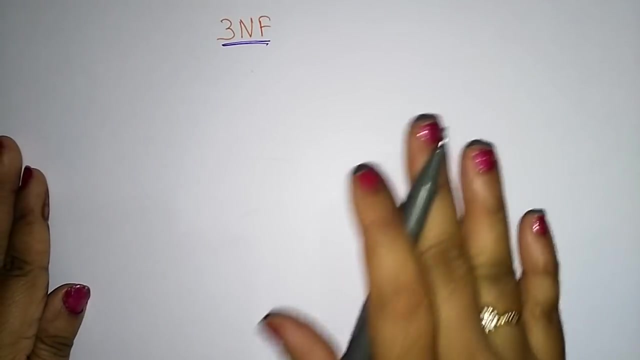 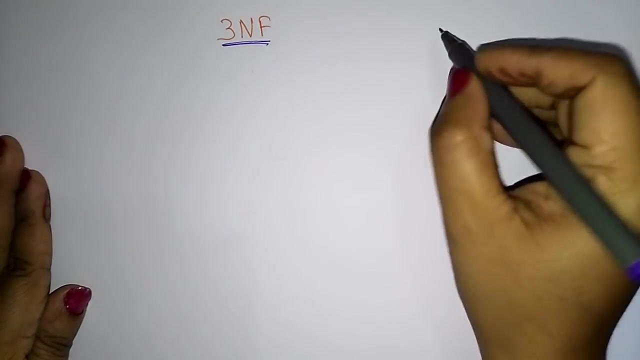 Hi students, coming to the next topic in the subject, database management system, is 3NF. In the previous videos I explained about first normal form and the second normal form. Now coming to third normal form. So what is this 3NF? So actually, in 3NF, all non-key attributes of a table must be functionally dependent on candidate keys. That is suppose if you take any table, so a table consisting of set of attributes. 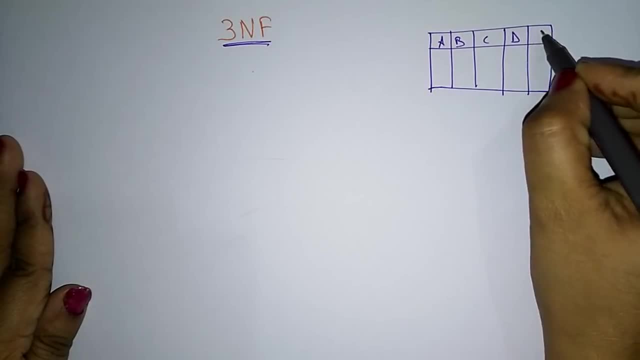 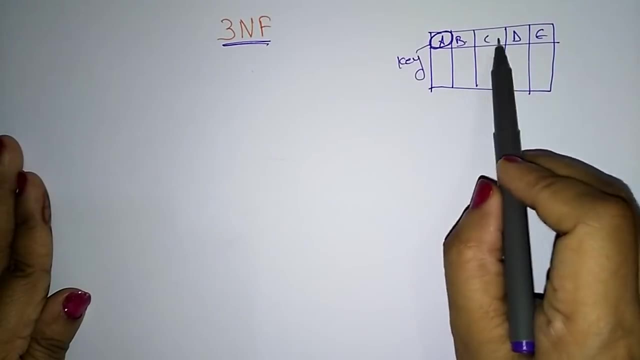 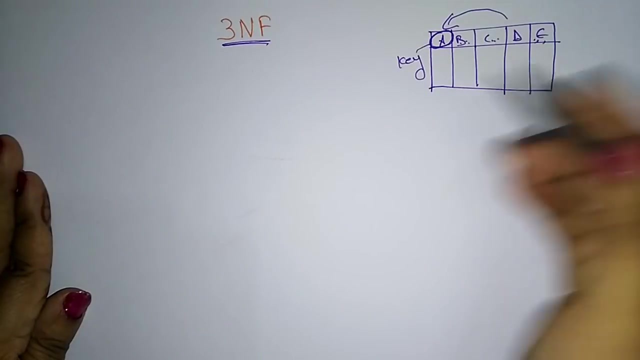 So these are the attributes. So here let's take this as a key key attribute. So this- the remaining items are called as a non-key attributes. So here in 3NF all non-key attribute must be functionally dependent on a candidate key, or else you can see that. 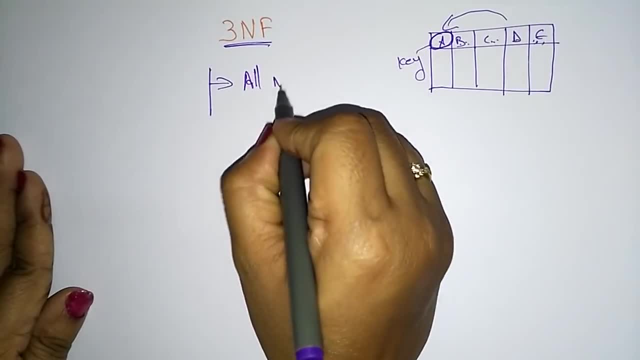 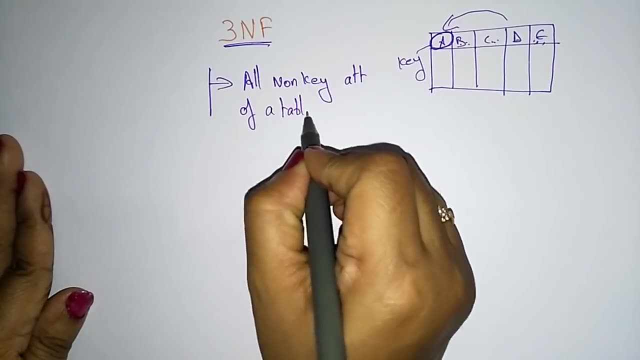 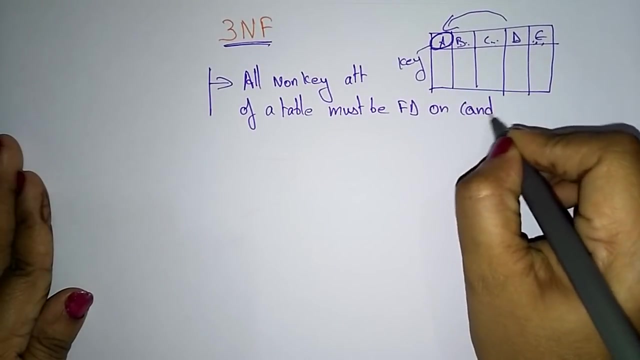 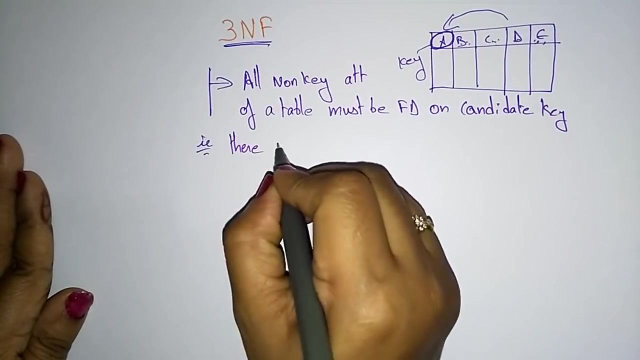 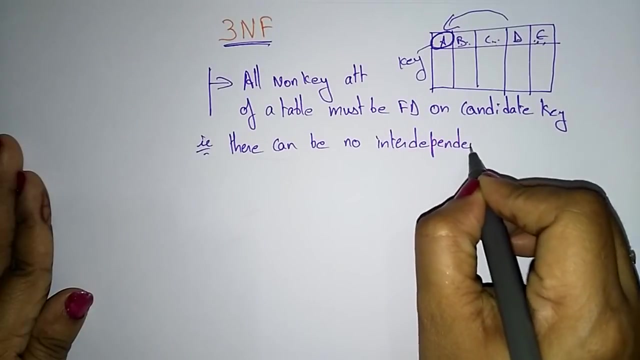 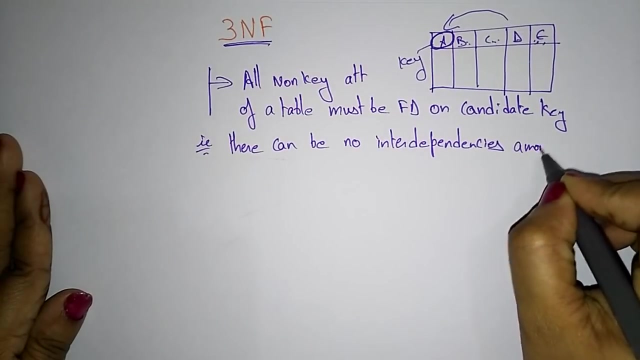 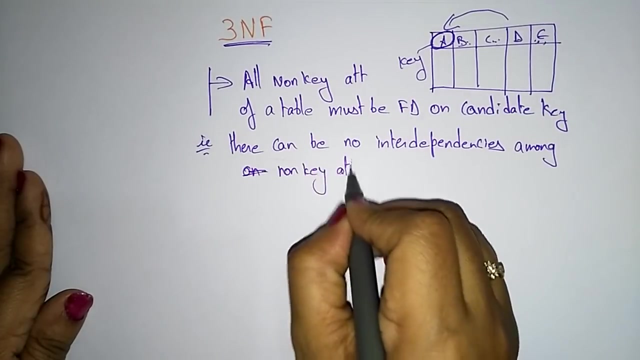 First, let me write that point: All non-key, All non-key attributes of a table must be functionally dependent on candidate key. That is, there can be no interdependency, Interdependencies, No interdependencies among, among non-key attributes, Among non-key attributes. 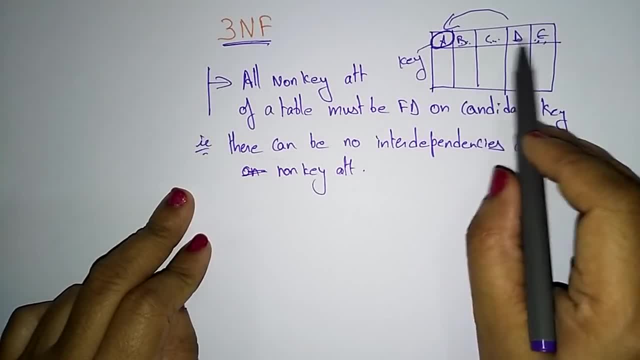 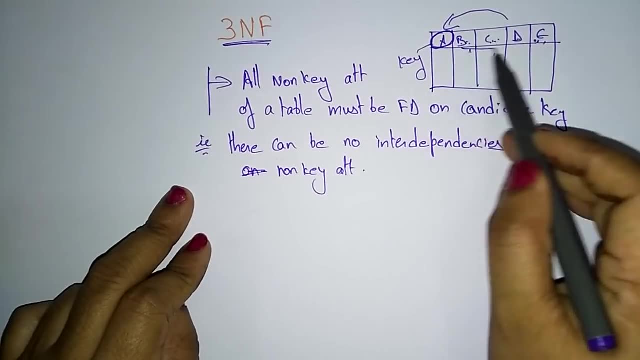 So here there can be no interdependency. So these are the non-key attributes. There can be no interdependency among these non-key attributes. Only all these non-key attribute must be functionally dependent on a candidate key. So if any 3NF. 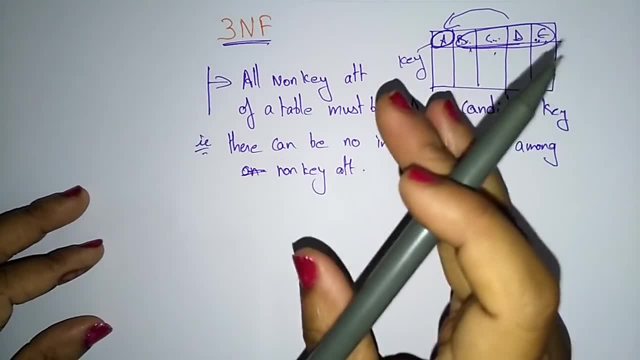 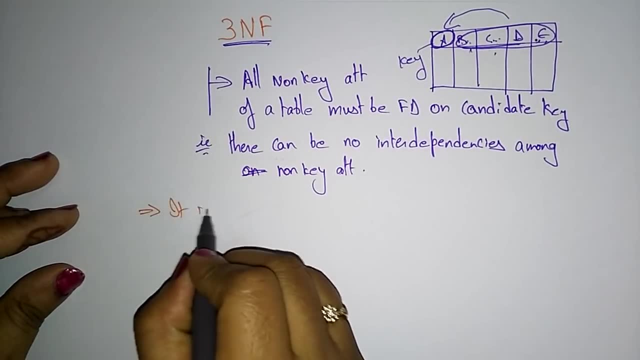 If a third, A third normal form must be in 3NF means it has to follow some points. That is, a 3NF should be. It is in 2NF. So the first is the table should be converted into 2NF. 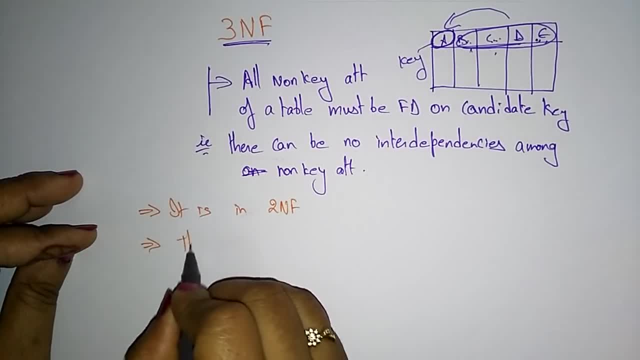 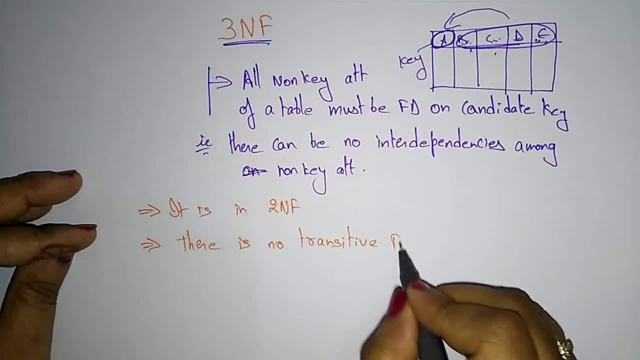 Second, normal form. And next, there is no, There is no transitive function dependency. So the one thing you have to be remember that, So the one thing you have to be remember that, So the one thing you have to be remember that 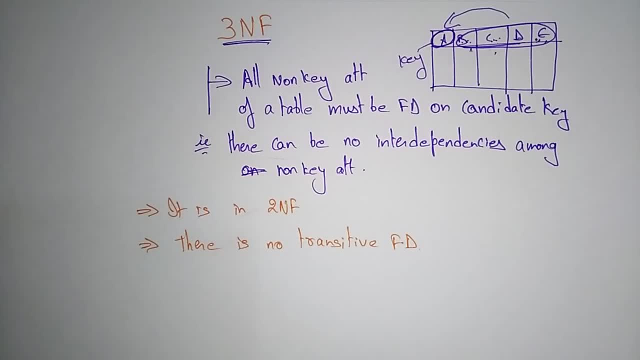 In the third normal form, The first, you have to convert that table into second normal form And there is no transitive functional dependency. So what is a transitive functional dependency? If A determines B, B determines C, Then A should determine C via B. 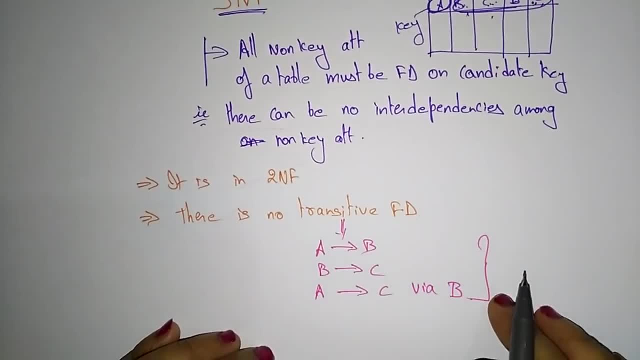 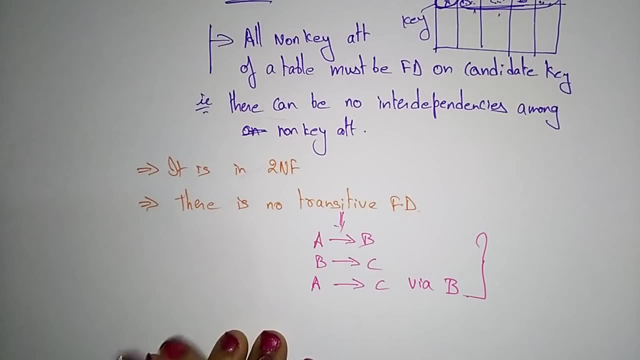 This is a transitive dependency formula. Okay, So this condition is not exist In the 3NF, So the 3NF. there is no transitive functional dependency. So whenever, if table is in, this Is following the transitive functional dependency. 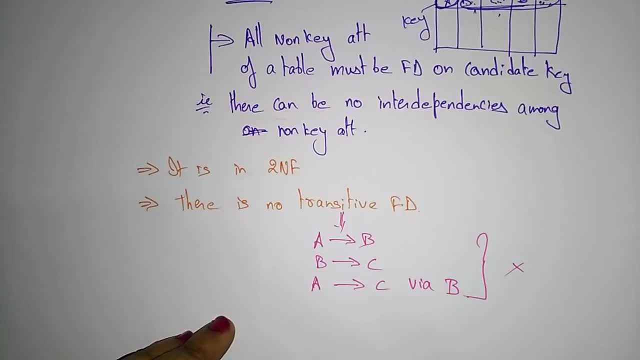 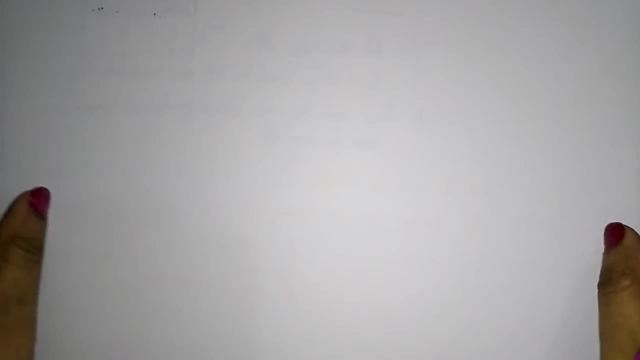 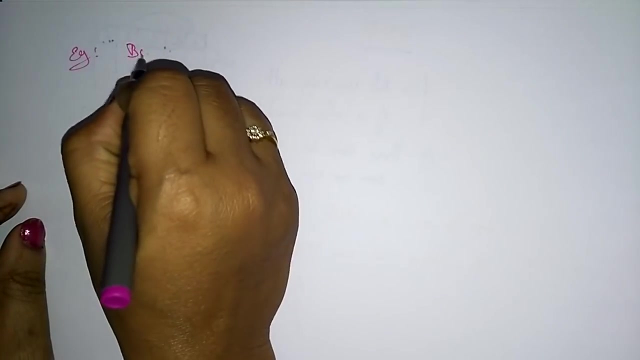 You have to convert that table into Non transitive dependency. Let me take some example, Then you will clearly understand How I am dividing the table, Converting the table into 3NF. Let me take one example. Let take, Let take book details. 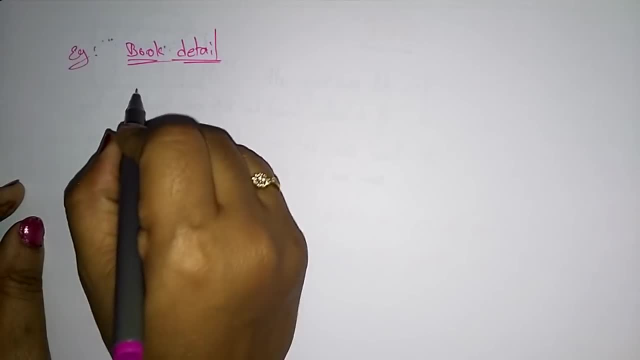 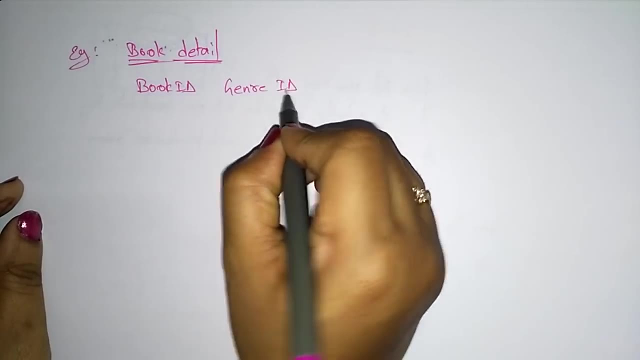 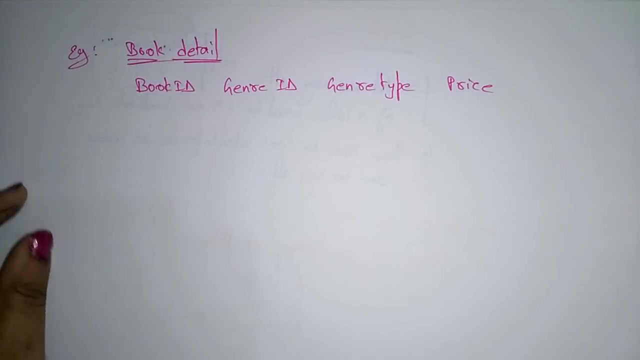 Book detail: Okay So book ID, Book ID And a Gener ID And gener type And the price. Okay, So these are the attributes that were present in the table And let me take the fields for this all: 1,2,3,4,5.. 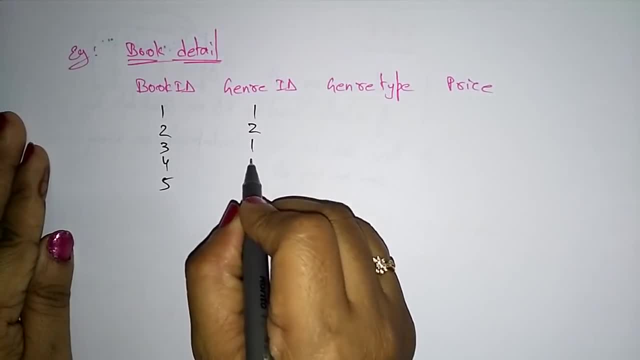 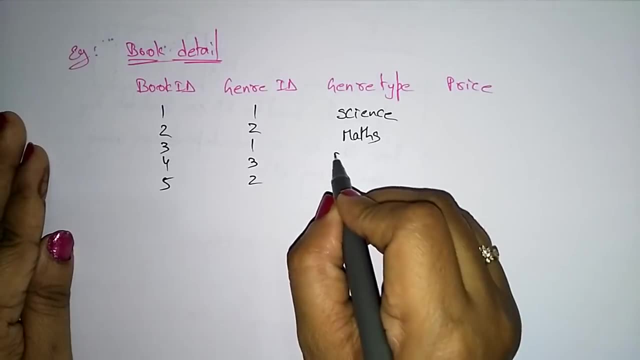 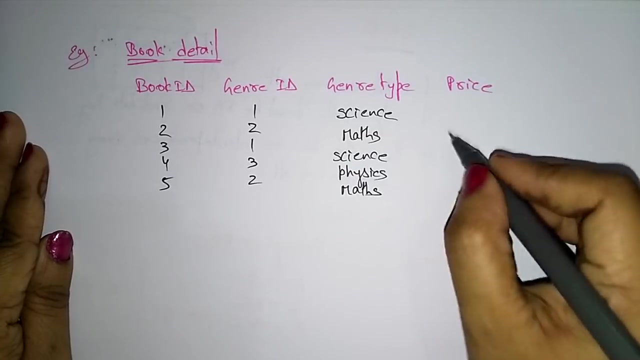 And the gener ID I am taking 1,2,1,3,2.. And the gener type is Science, Maths, Science, Physics And Maths. Okay, And the prices for those are suppose 30,35.. 25,20,30.. 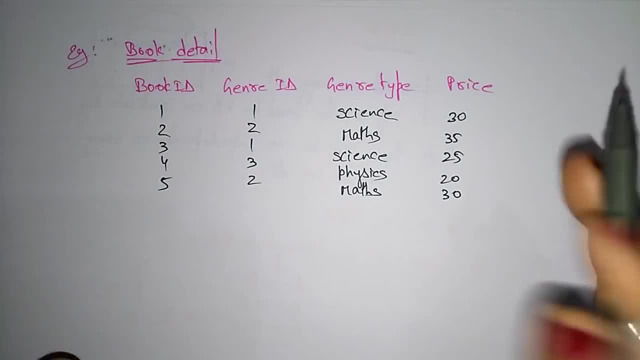 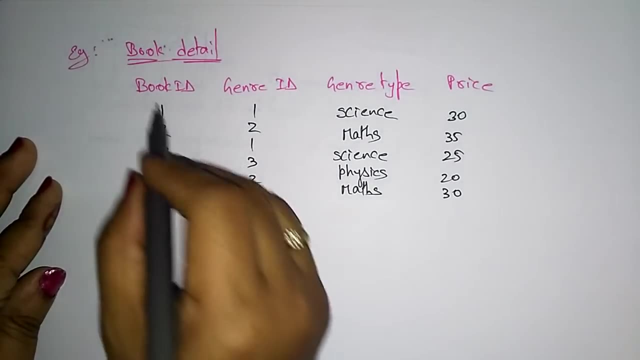 So these are the prices for these books. Okay, So this is a table Which is Not in 3NF. How can I say this is not in 3NF? Because Here This book ID. So this is a book ID. 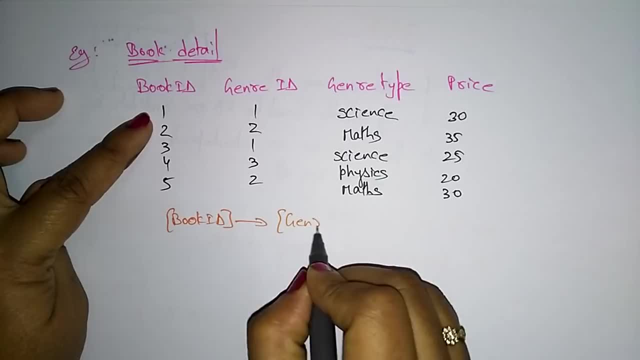 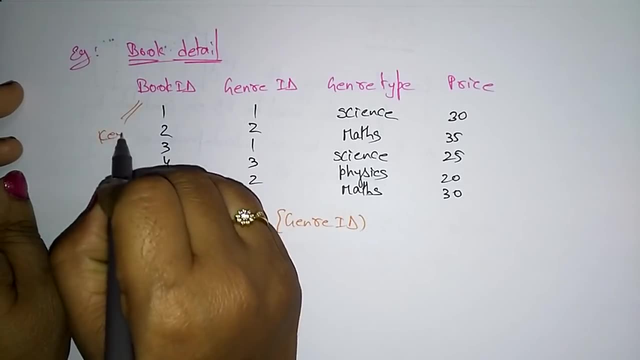 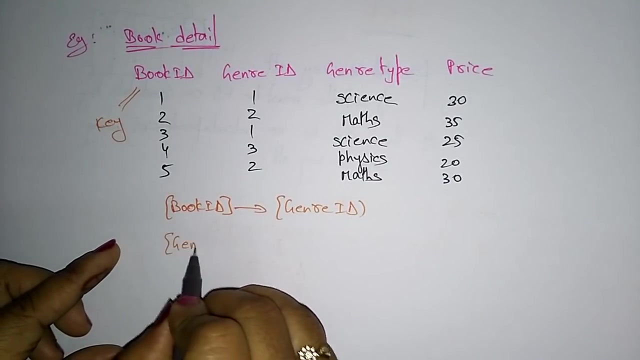 This book ID determines the Gener ID, Because this is a unique value. So this I am taking it as a Key attribute. So this book ID is a key attribute. So book ID determines the Gener ID And the gener ID. 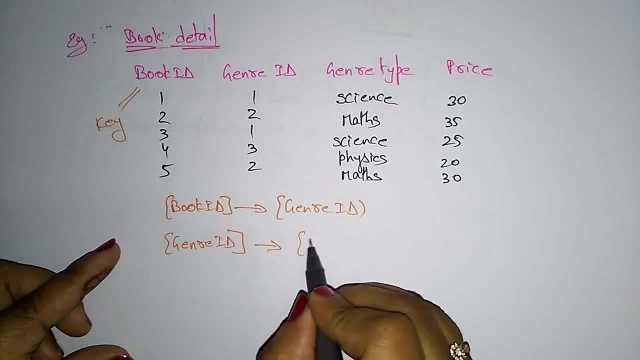 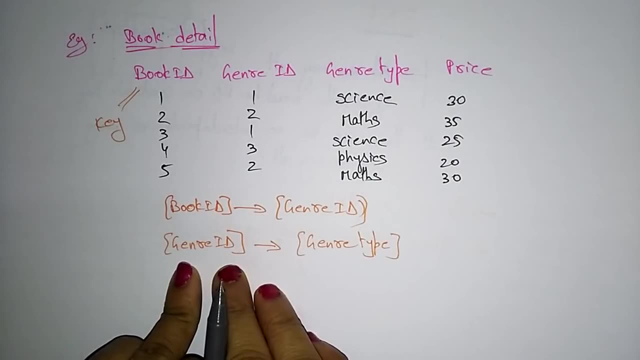 Gener ID. Gener ID determines the Gener Type. Gener type means Here: the gener type is functionally dependent on the gener ID And the gener ID is functionally dependent on book ID. Okay, And the book ID. This book ID is: 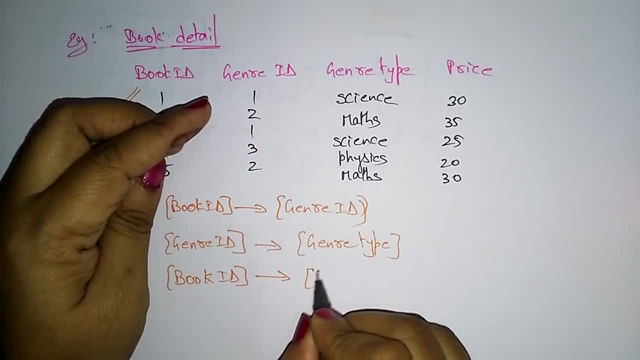 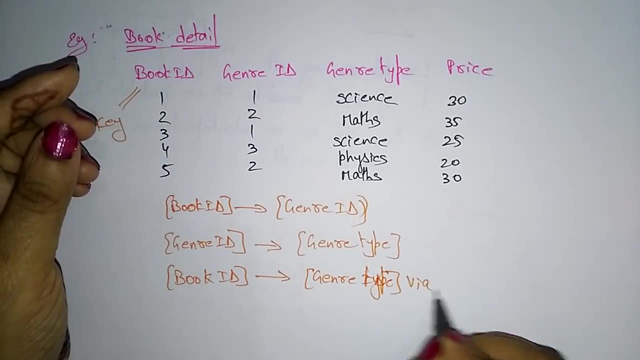 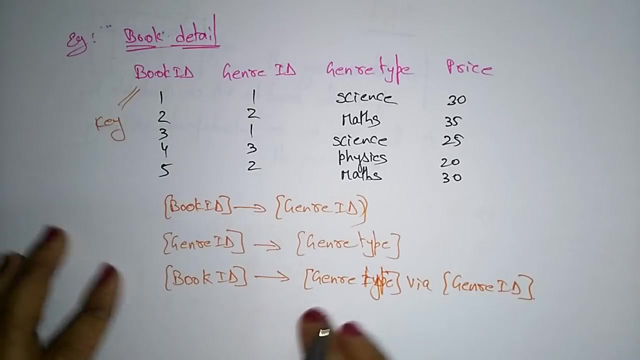 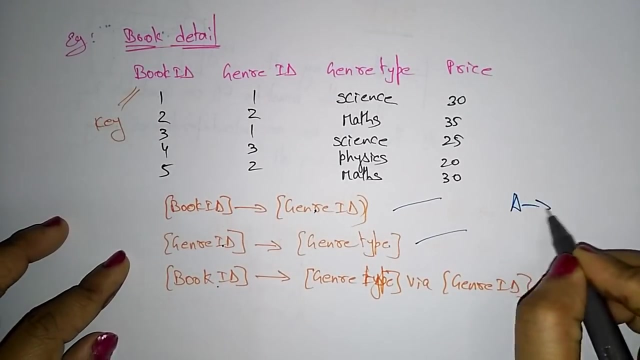 Determines the Gener ID, So gener type via general ID. So this table is following these conditions. So here the book ID determines general ID. general ID determines general type. book ID determines general type via general ID. It looks like A determines B. 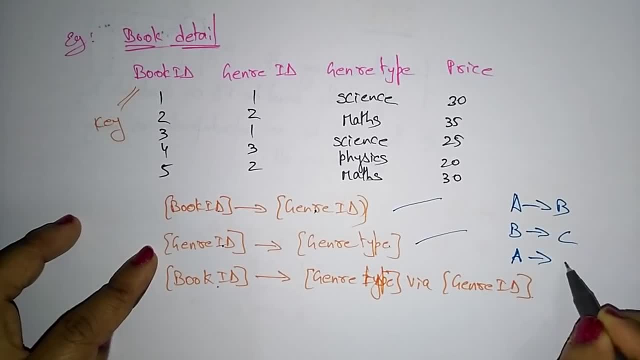 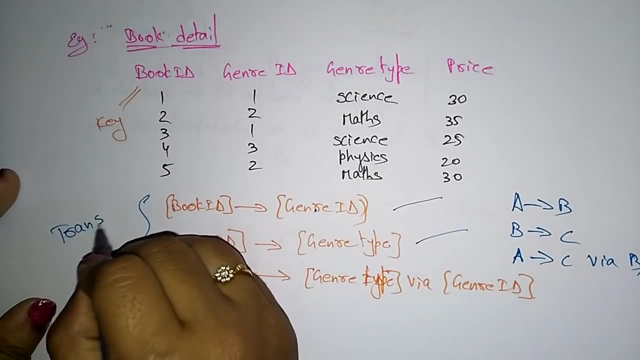 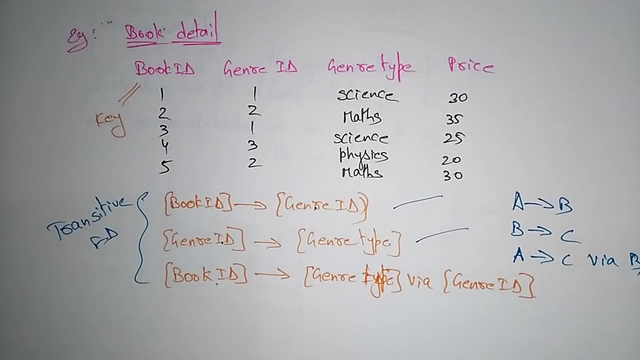 B determines C and A determines C via B. So this table is in. transitive dependency means existing transitive functional dependency. So now I want to make this table to 3NF. So let decompose this table. Decompose. 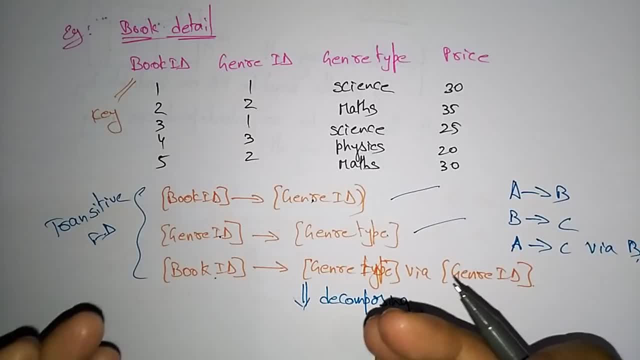 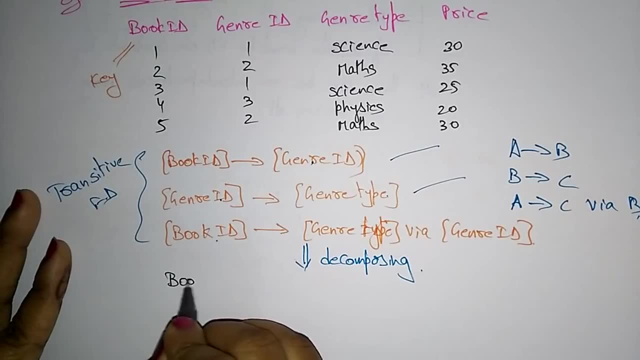 Decomposing this table. So I am just dividing this table to make it this table as a 3NF. So I am taking 2NF. So here I am taking book 1 table and general ID is general is 1 table. 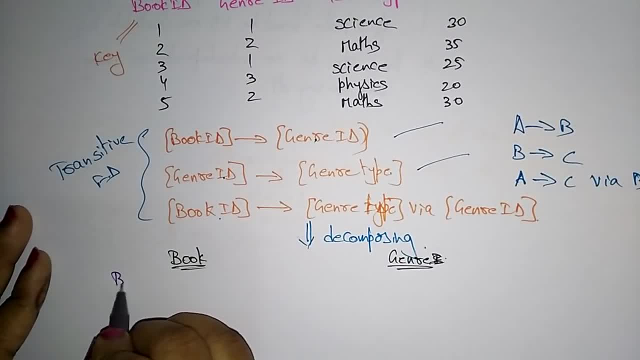 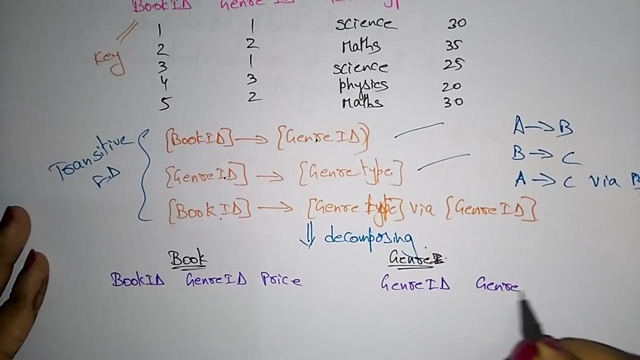 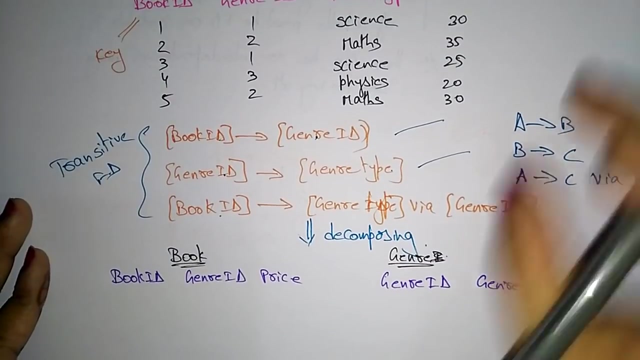 And the fields for this tables are book ID, general ID and the price. And the fields for this general table are general ID and general type. So here I am just decomposing this table into 2 tables So that the table will satisfy the 3NF condition. 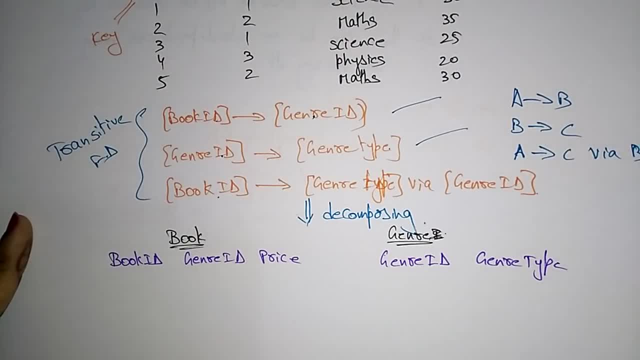 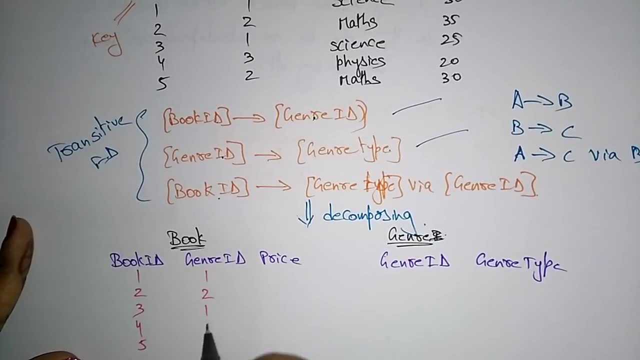 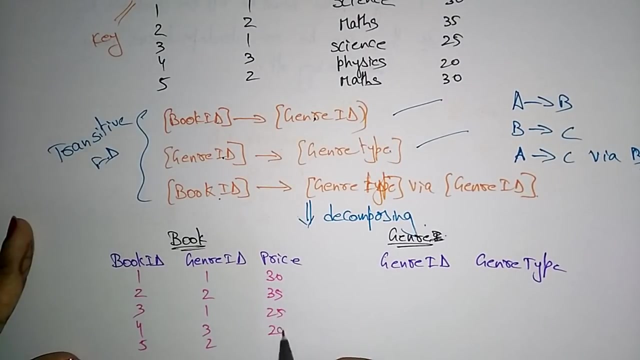 So here the fields for this are book ID 1, 2, 3,, 4, 5, and the general ID is 1, 2, 1, 3, 2.. And the relating price for those books is 25, 20, 30.. 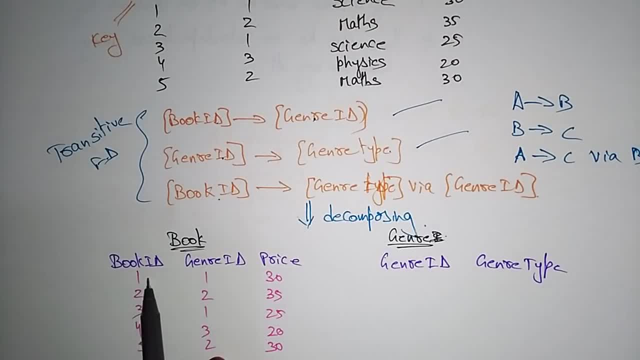 So here you can observe that the book ID determines general ID. Okay, So the book ID determines here. this book ID is a primary key. Let's take this as a primary key. So here the now all non-key attributes. What are non-key attributes? general ID and the price. 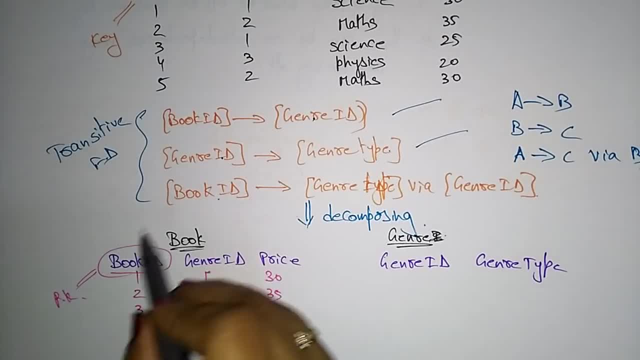 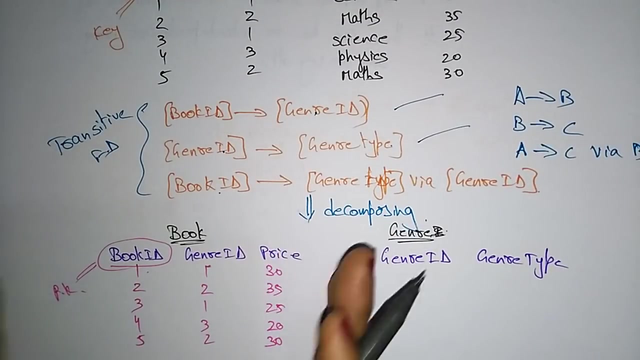 So these non-key attributes are fully functionally dependent on the primary key. So both general ID and the price Depends upon the book ID. So it's satisfying the first condition, that is, it is in 2NF. Okay, It is in 2NF and there is no transduce functional dependency on this table. 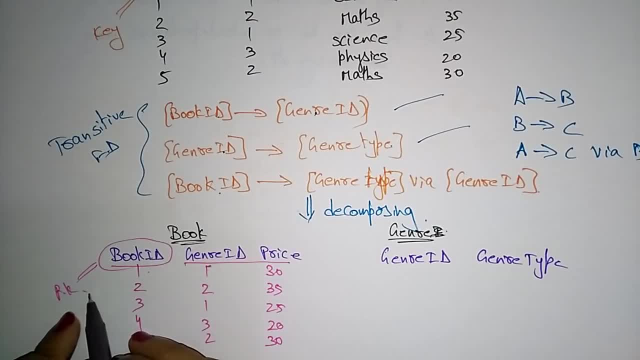 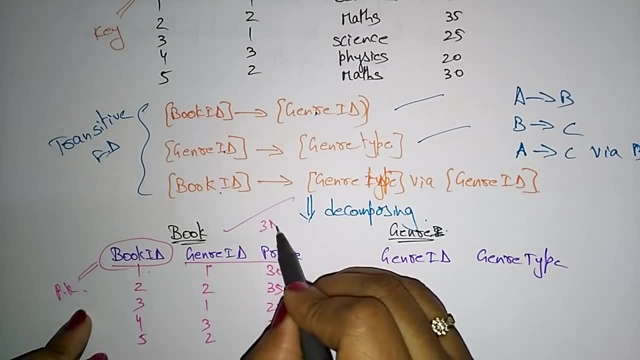 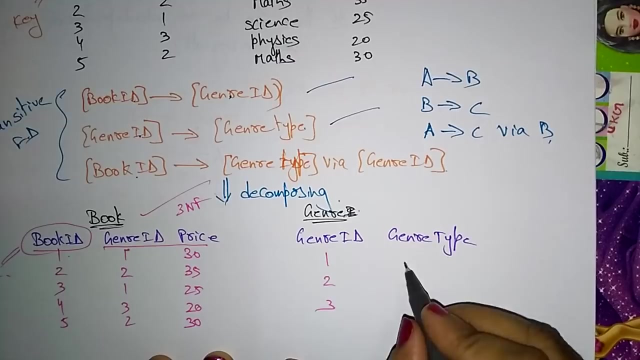 Because all non-key attributes is depends upon the fully functional, depends upon the primary key attribute. Okay, This table is in 3NF And the same way here also. the general ID is 1,, 2., 3. And for 1 it's having 1 is signs. 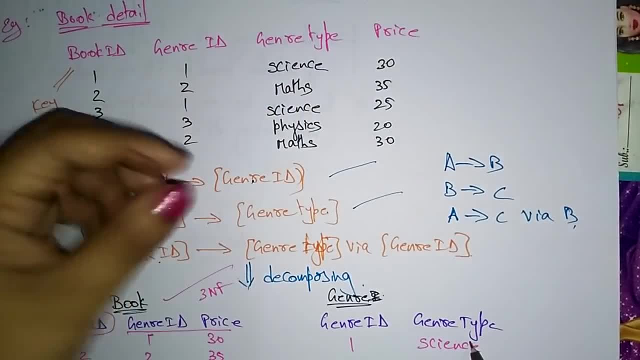 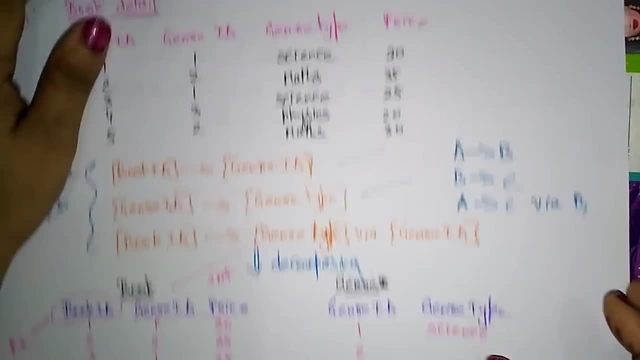 Here also, the 1 is signs, So we are taking only 1 value because it eliminates the redundancy. The main aim of this third normal form is to eliminate the redundancy. And 2 is. here you are having the 2 general IDs, 2 numbers, and they are related to max. 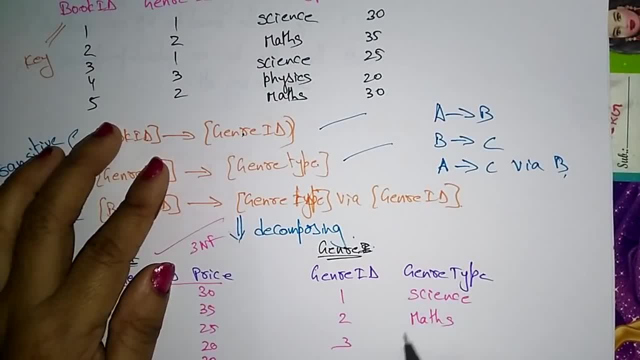 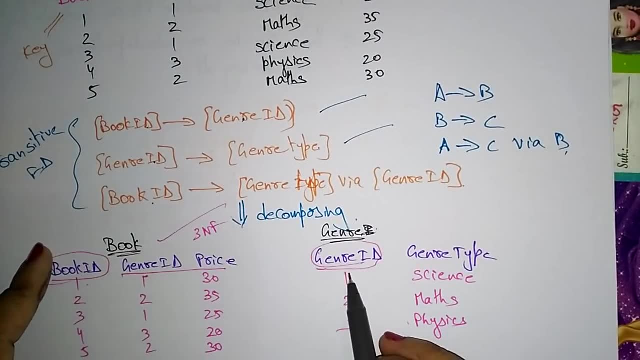 So just write 1 max for general ID 2. And 3 is physics. So here this is In this table. this is acting as a key attribute, Okay, And this is a non-key attribute. The non-key attribute is fully functionally dependent on the key attribute. 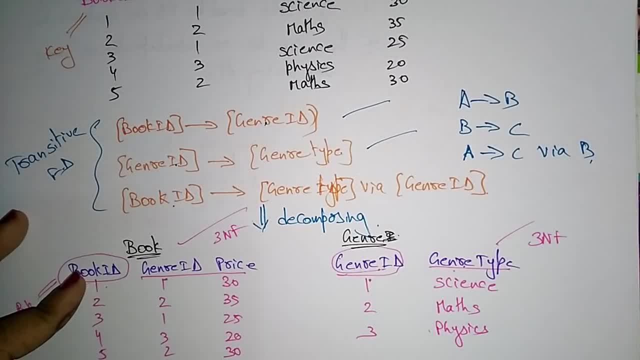 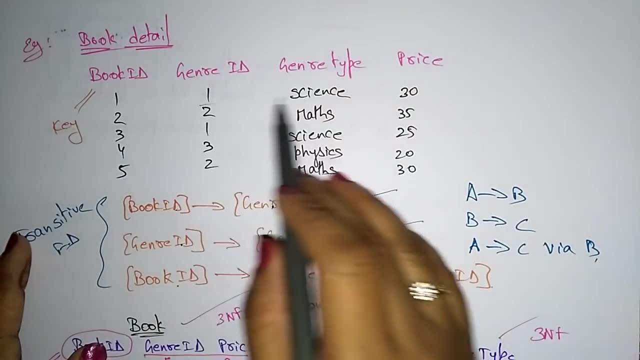 So this is also in 3NF. So this is how you have to decompose the table. So, whatever the table that is there, which is having the redundant data, So this is the redundant data. So, which is having the redundant data? 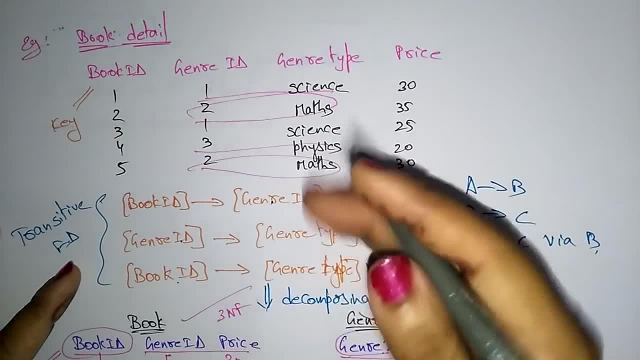 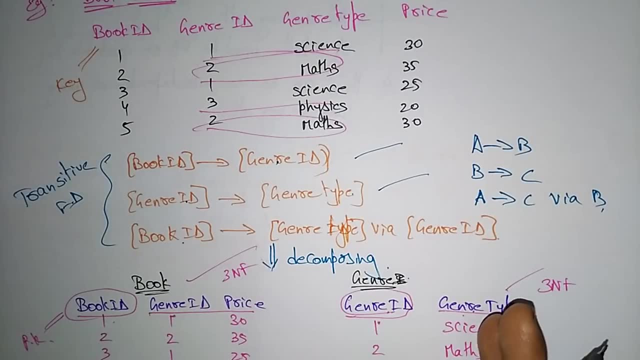 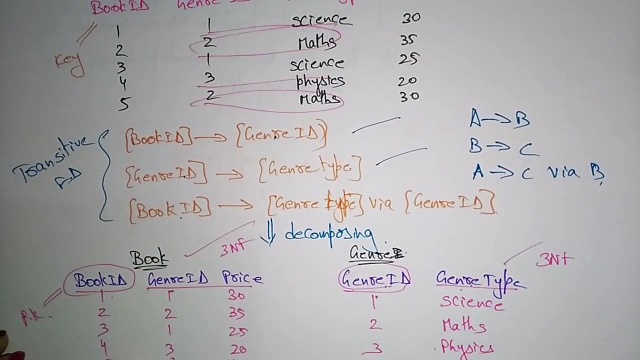 Okay, So that data. So that data. To eliminate this redundancy, we are decomposing this table into 2 tables So that the redundant data will be eliminated And also it follows the conditions that all the non-key attributes is fully functionally dependent on the primary key. 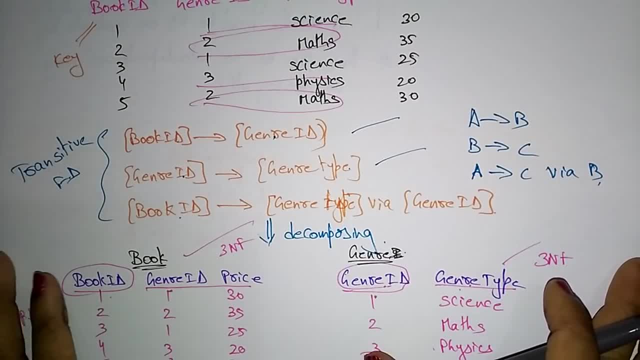 And here there is no transitive dependency will be existed. Okay, So this is about the 3NF, Thank you.